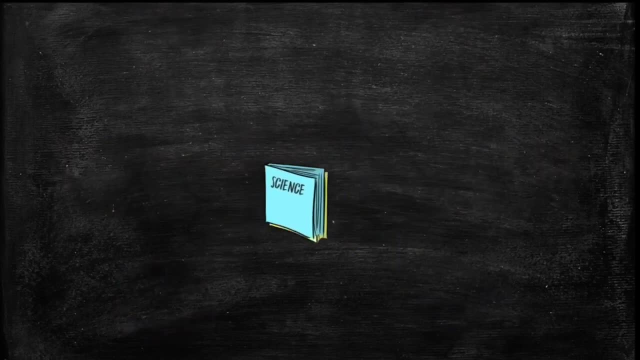 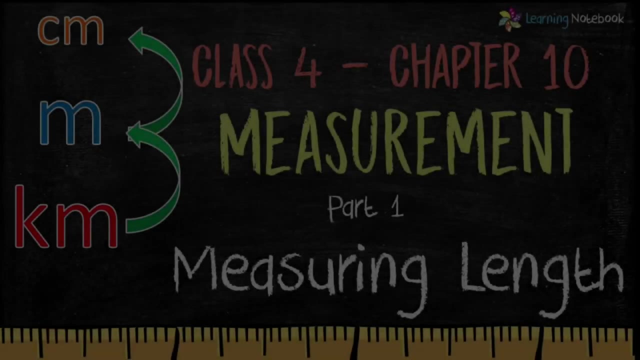 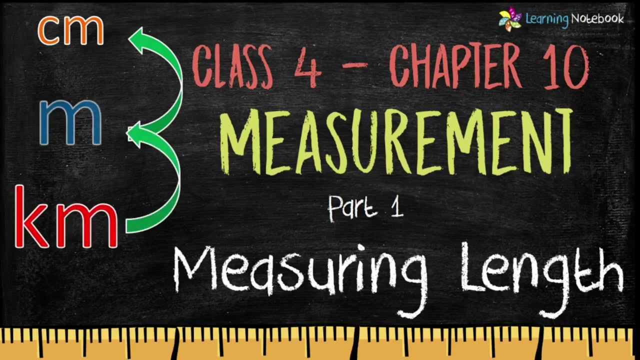 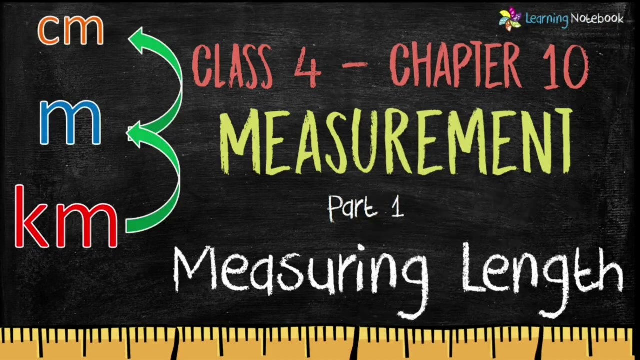 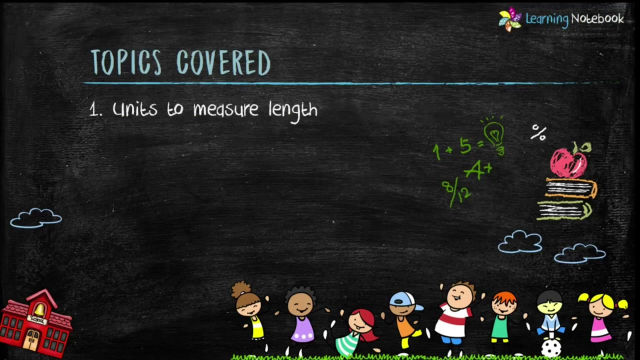 Hello students, welcome to our channel Learning Notebook. In today's video we will do part 1 of chapter Measurement. In this part 1, we will understand measurement of length. So let's start and see what all topics we are going to cover today. 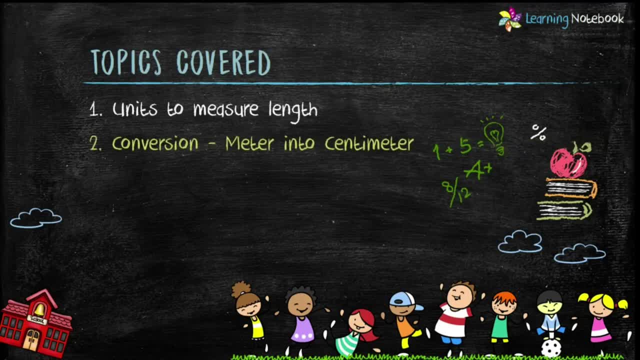 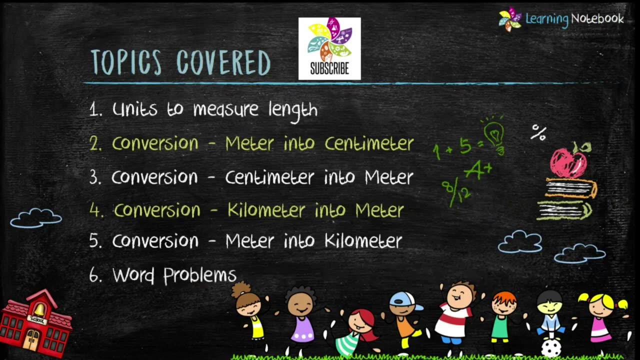 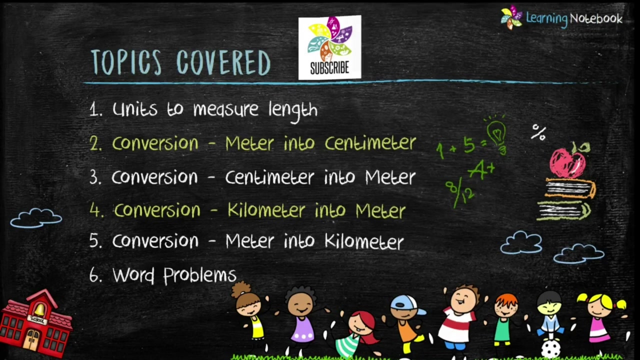 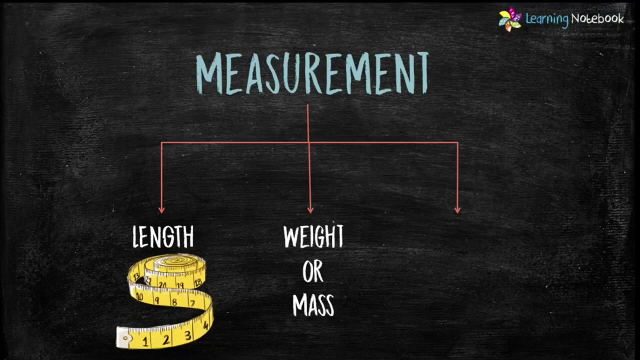 First is Units to measure length. Second, conversion of meter into centimeter, After that centimeter into meter, kilometer into meter and meter into kilometer. In the end we will solve few word problems. Students, when we talk about measurement, we talk about measurement of length measurement. 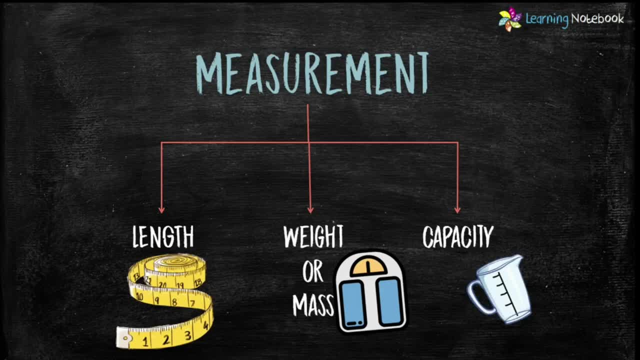 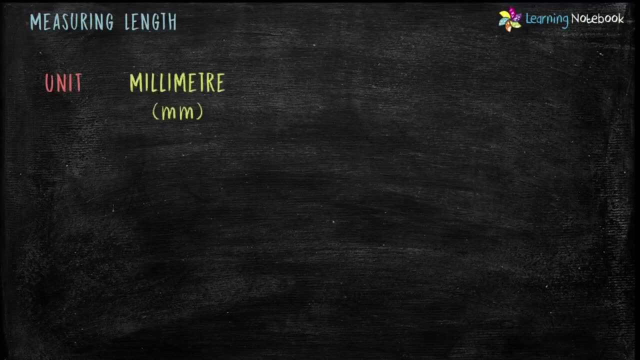 of weight or mass and measurement of capacity. In part 1 and part 2, we will do measurement of length. Let's first see the units to measure length. First unit is millimeter, which is denoted by mm. Millimeter is used to measure very 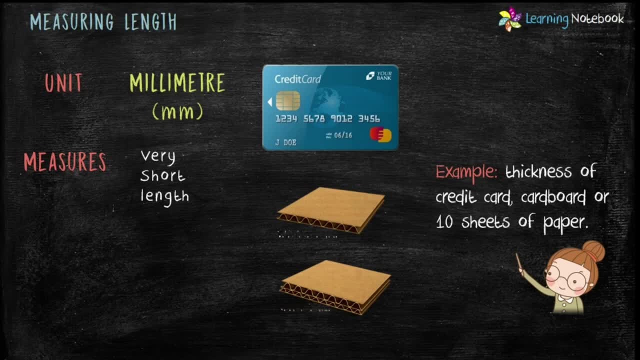 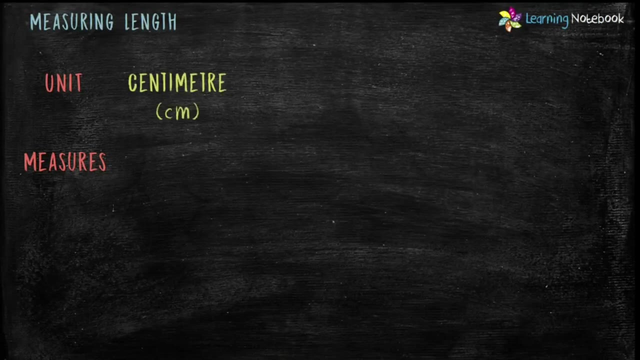 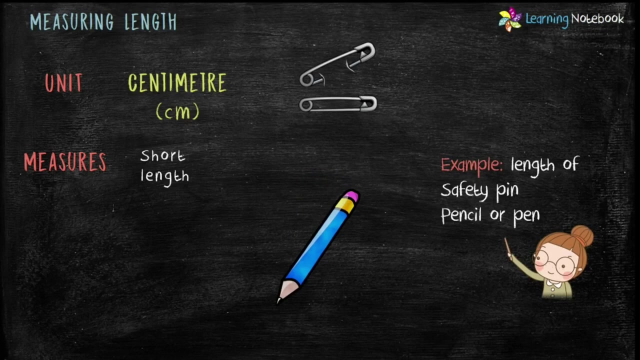 short length. For example, we can use millimeter to measure thickness of credit card cardboard or 10 sheets of paper. Second unit is centimeter, which is denoted by cm. Centimeter is used to measure short length. For example, we can use centimeter to measure. 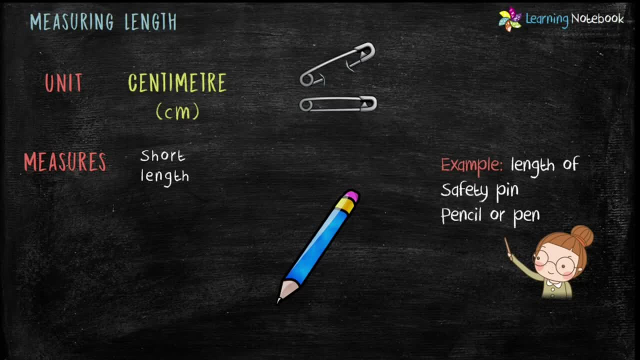 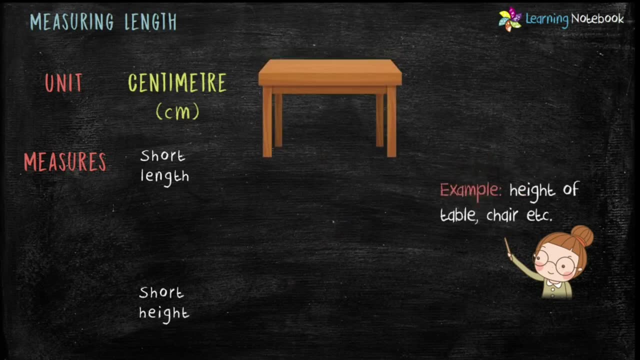 length of safety pin, pencil or pen Students. centimeter is also used to measure short height. For example, height of table chair, etc. can be measured using centimeter. Andρό is used in world exam to measure height. 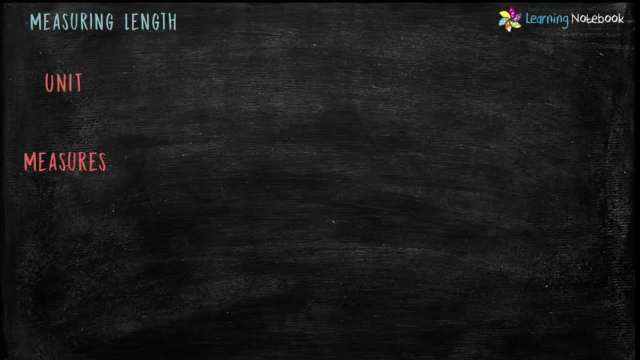 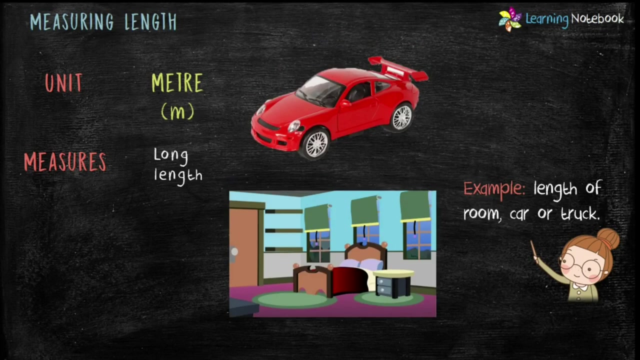 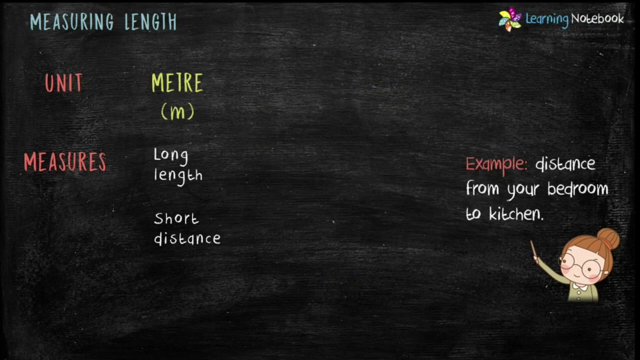 centimeter. Next unit of measuring length is meter, which is denoted by M. Meter is used to measure long length, like length of room, car or truck Students. meter is also used to measure short distance. For example, distance from your bedroom to kitchen is measured in meter and meter. 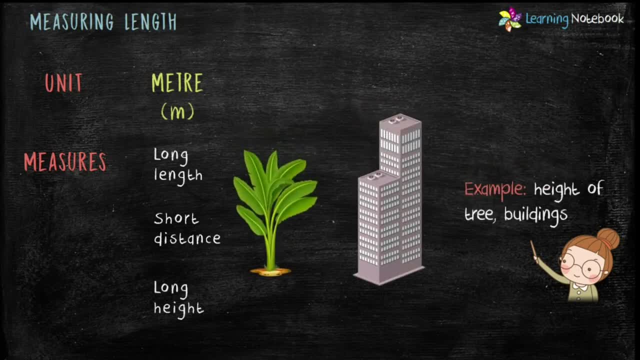 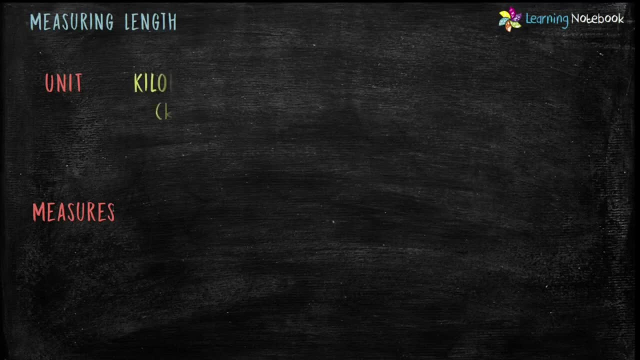 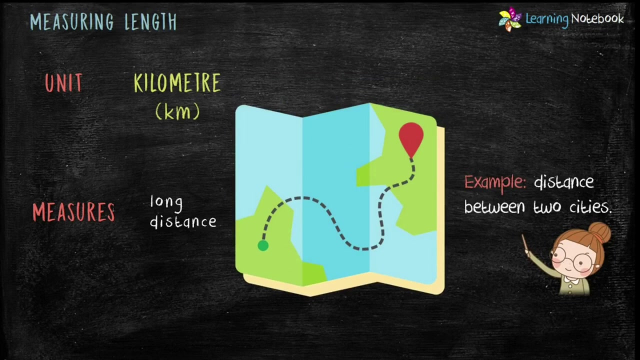 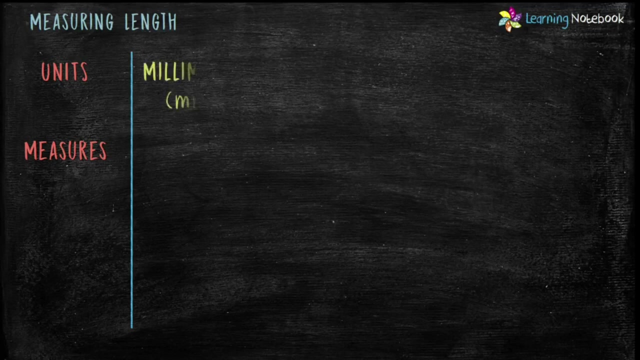 is used to measure long height, like height of tree or height of buildings. Last unit is kilometer, which is denoted by KM. Kilometer is used to measure long distance. For example, distance between two cities is measured in kilometer. Students, let's summarize. 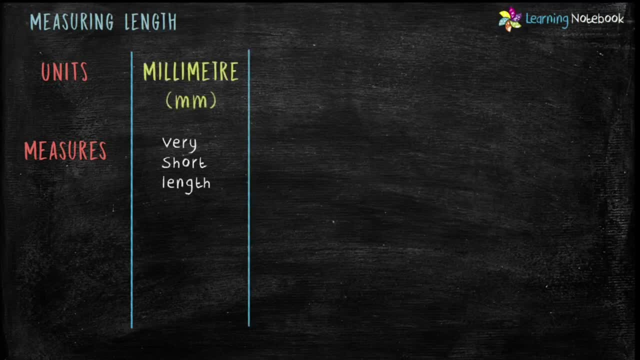 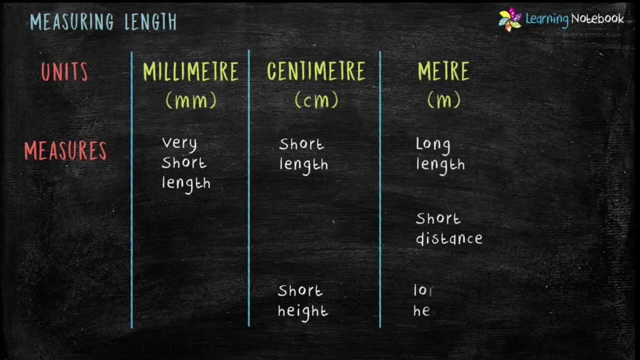 the four units to measure length. First is millimeter, which is used to measure very short length. After that centimeter, which is used to measure short length and short height. Third is meter, which is used to measure long length, short distance and long height. And the last one is: 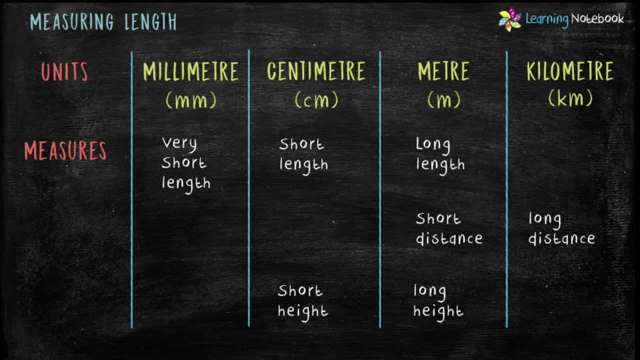 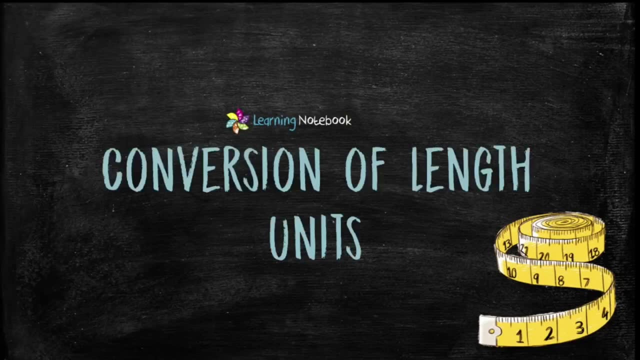 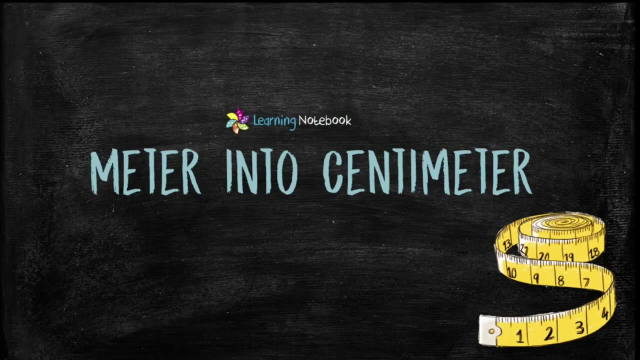 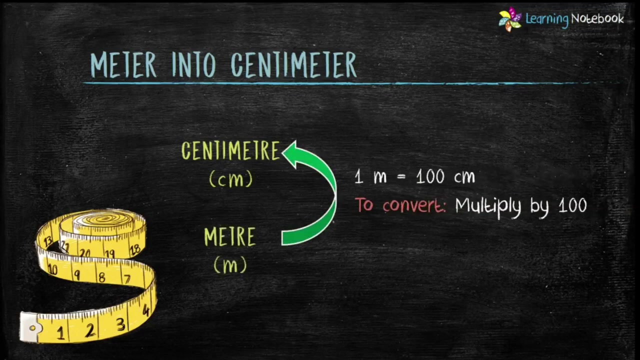 kilometer, which is used to measure long distance. So now let's see how to convert these length units. First is meter into centimeter. 1 meter equals to 100 centimeter, So to convert meter into centimeter, multiply by 100.. Let's see. 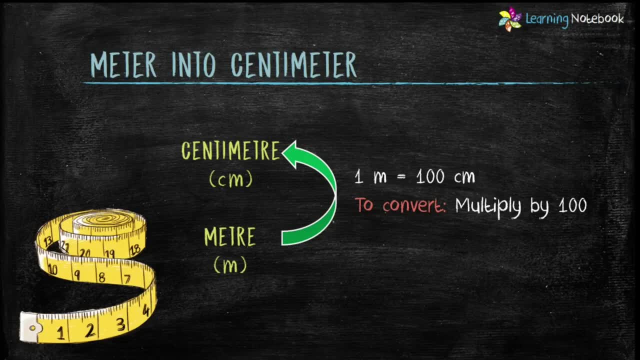 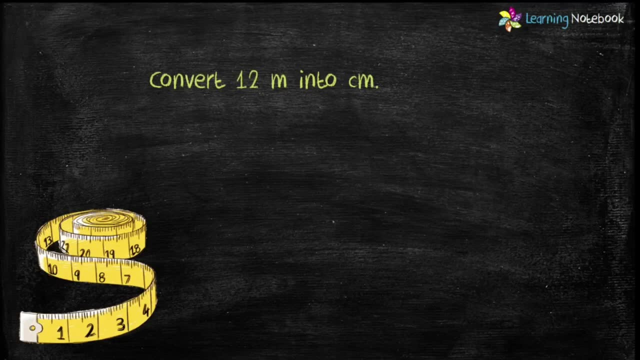 few examples to understand the same. First example is: convert 12 meter into centimeter. I just told you 1 meter equals to 100 centimeter. I just told you 1 meter equals to 100 centimeter. I just told you 1 meter equals to 100 centimeter. Therefore, to convert 12 meter into centimeter, we will. 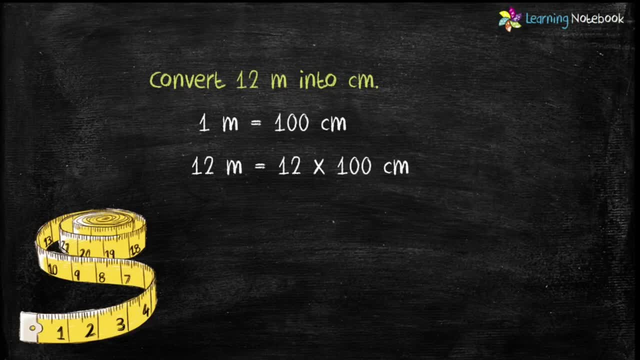 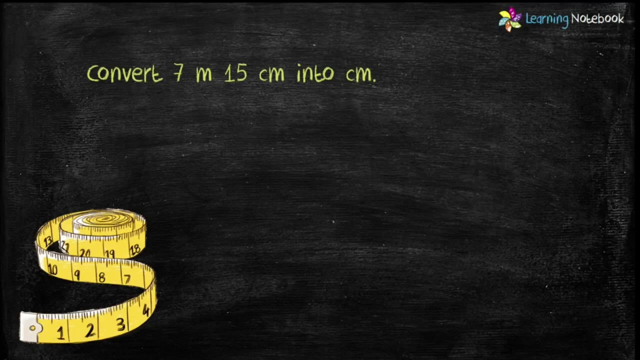 multiply 12 with 100, which is equals to 1200 centimeter. So, student, 12 meter equals to 1200 centimeter. Let's do one more example: Convert 7 meter 15 centimeter into centimeter. 7 meter 15 centimeter means 7 meter plus 15 centimeter. Now we have. 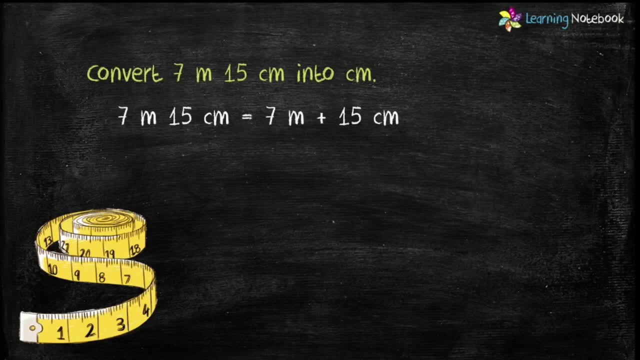 Now we have 2 terms: 7 meter and 15 centimeter. Now we have 2 terms: 5 meters, 12 meter and 15 centimeter. 15 is already in centimeter, So let's convert 7 meter into centimeter. To convert 7 meter into centimeter, multiply: 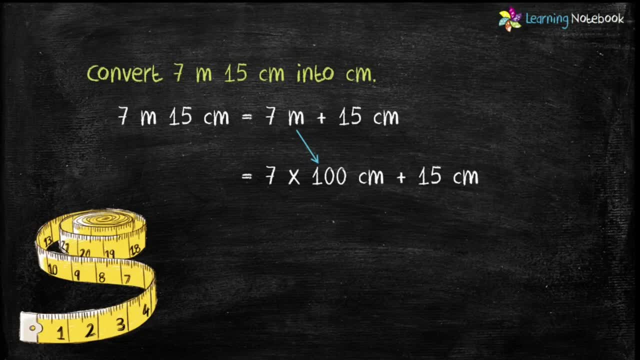 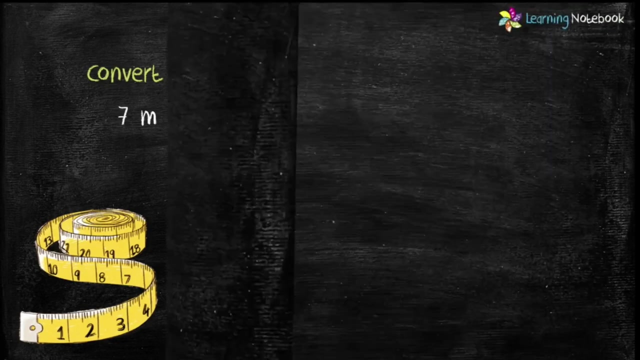 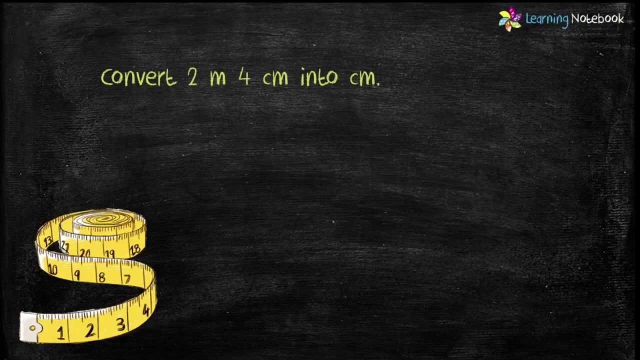 you multiply 9 plus 10 power 0, which 7 x 100 cm. 7 x 100 equals to 700 cm. Therefore, 700 cm plus 15 cm equals to 715 cm. Let's see one more similar example: Convert 2 meter 4 cm into cm. Student, as I just told. 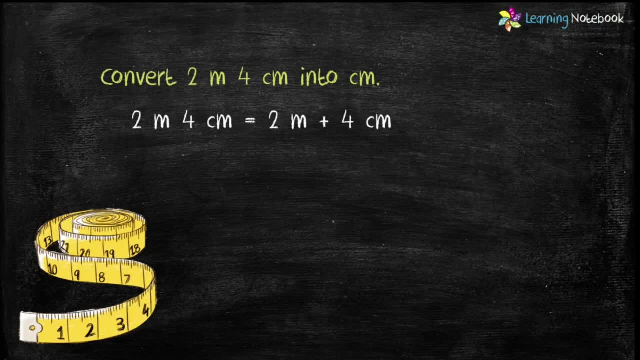 you 2 meter 4 cm means 2 meter plus 4 cm. 4 is already in cm. So now let's convert 2 meter into cm, which is equals to 4.. 2 x 100 cm, because to convert meter into cm we will multiply by 100.. Now 2 x 100. 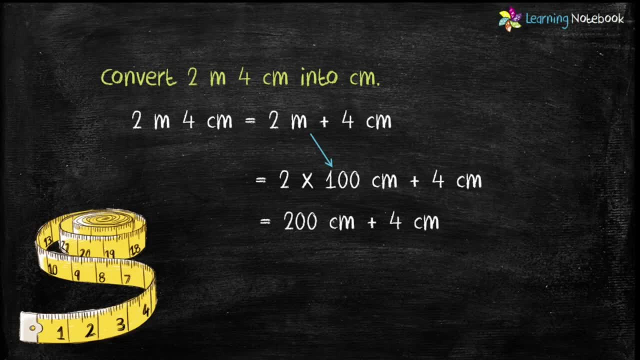 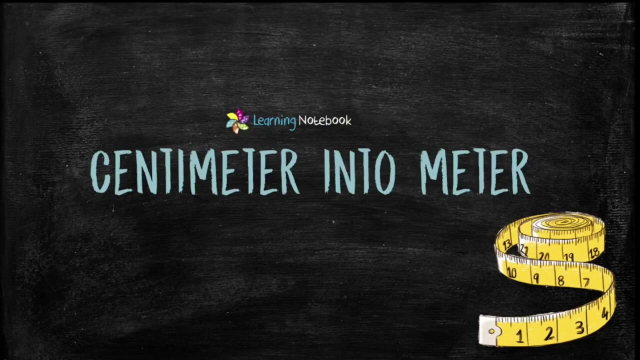 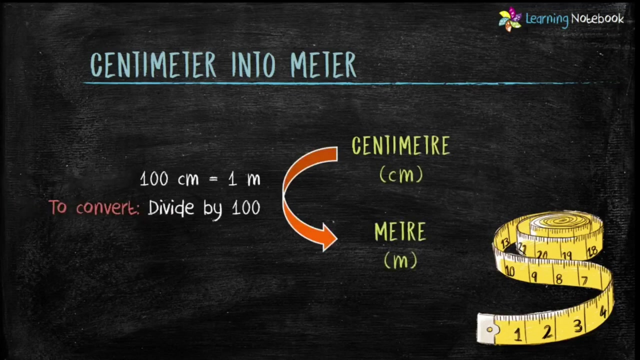 equals to 200 cm. Therefore, 200 cm plus 4 cm equals to 204 cm. So, students, this is how we convert meter into cm. Now let's see how to convert cm into m. Students, 100 cm equals to 1 m. So to convert cm into m, we will divide by 100. 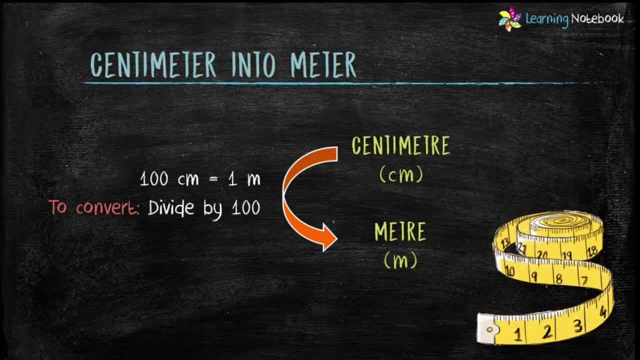 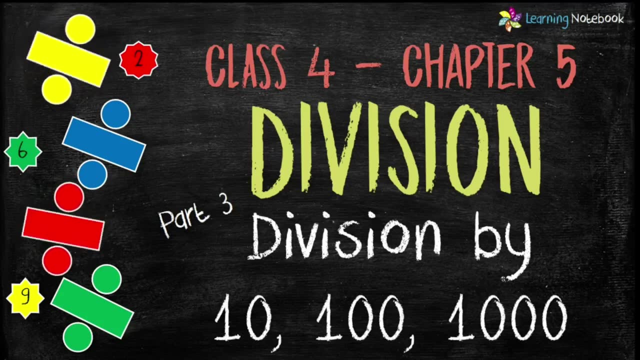 Let's solve few questions to understand this questions. first we need to understand division by 100.. We have already covered division by 10, 100 and 1000 in part 3 of chapter 5.. Students, make sure you watch this video. 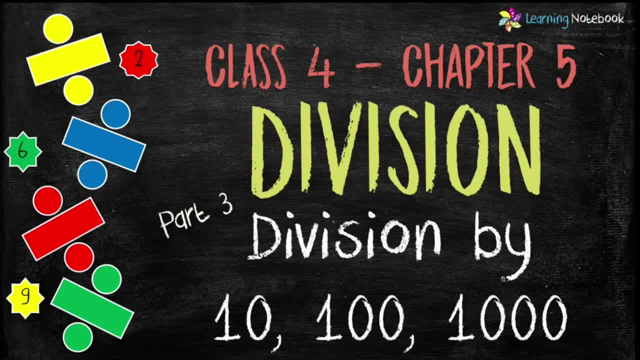 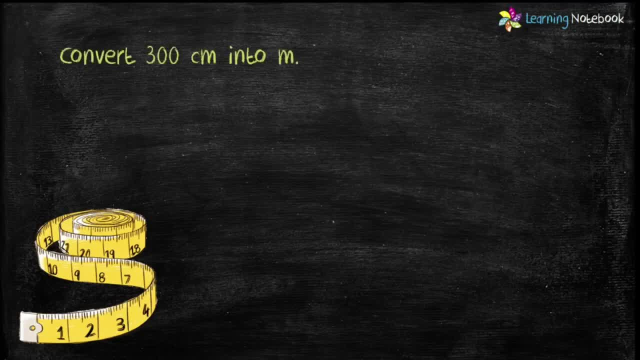 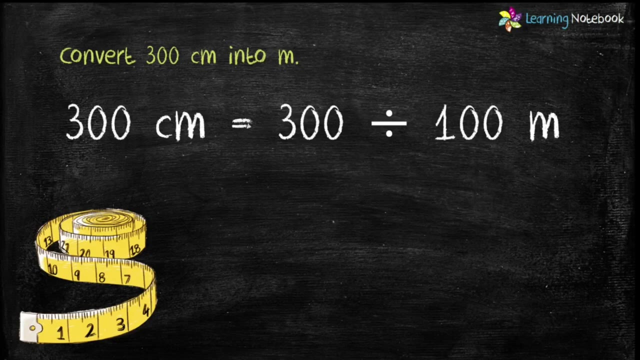 to understand how to divide without long division method. First question is: convert 300 cm into meter. Students, we just learnt to convert cm into meter. divide by 100. Therefore, 300 cm equals to 300 divided by 100 meter. And when a number 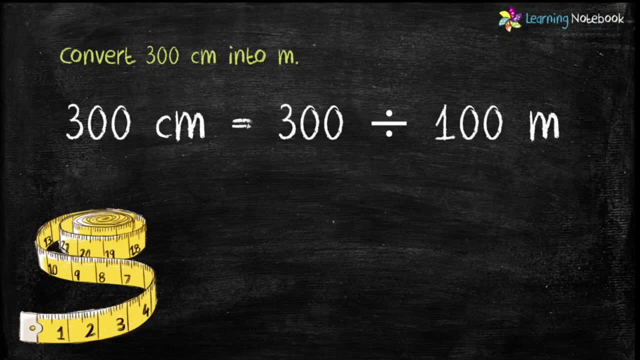 is divided by 100.. 2 digits at once in tenth place make up the remainder and rest of the digits make up the question. So in this case, remainder is 0 and question is 3.. Therefore our answer is 3 meter. 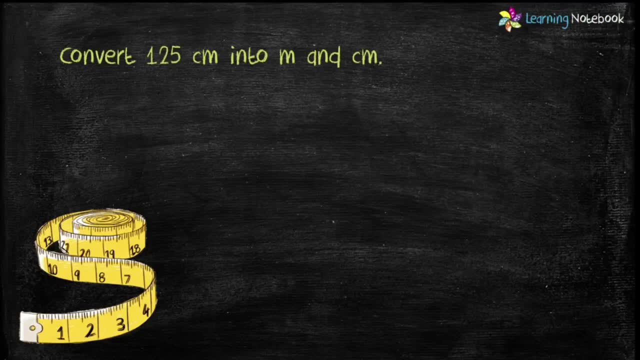 Second question is: convert 125 cm into meter and centimeter Again. students, to convert centimeter into meter, we will divide by 100.. And I just told you, when a number is divided by 100, digits at 1st and 10th place make. 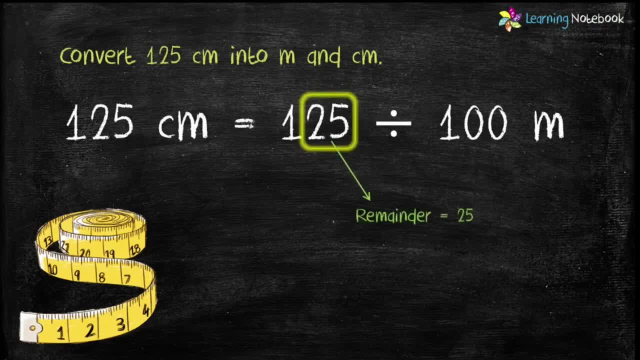 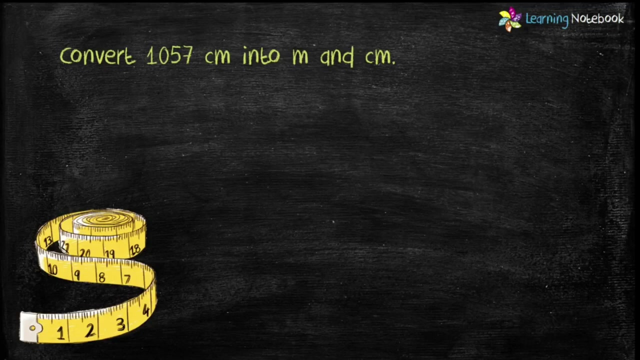 up the remainder. So here remainder is 25.. And rest of the digits make up the question. So here question is 1.. Therefore answer is 1 meter and 25 centimeter. Let's do one more question. Convert 1057 centimeter into meter and centimeter Students. 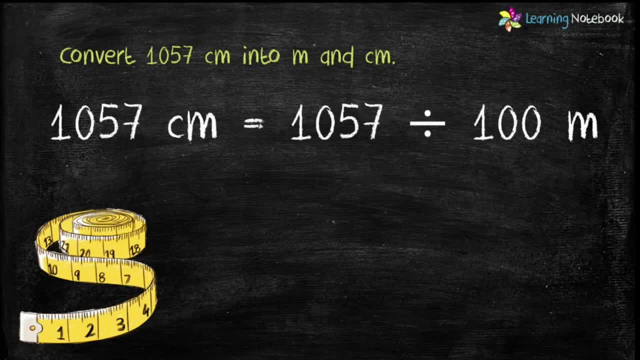 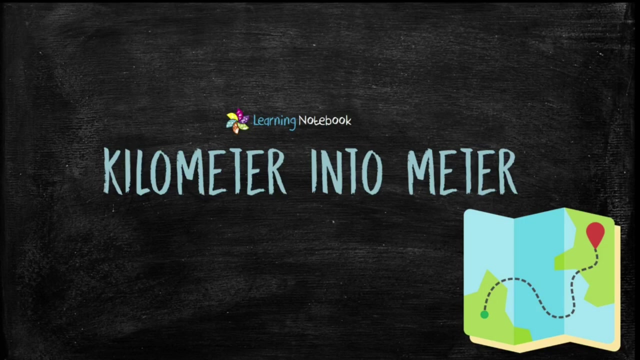 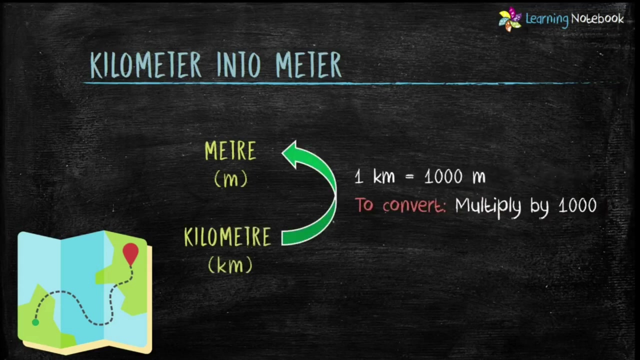 let's divide it by 100.. So here, 57 will be remainder And 10 will be question. Therefore, answer is 10 meter, 57 centimeter. Now let's see how to convert kilometer into meter. Students, 1 kilometer equals to 1000 meter. 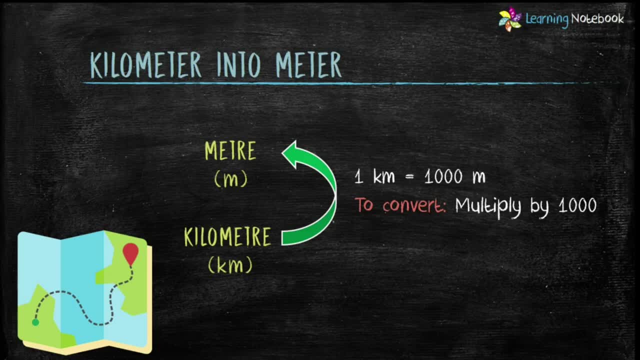 So, to convert kilometer into meter, we will divide by 100.. We will multiply by 1000.. Students, we have already done fractions, So can you tell me what will be half of a kilometer? Yes, it is 1000 divided by 2, which is equals to 500 meter. 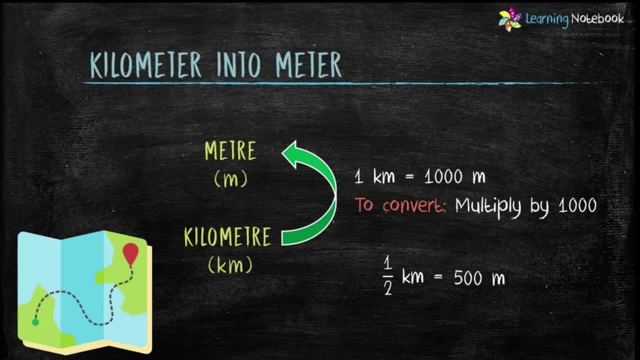 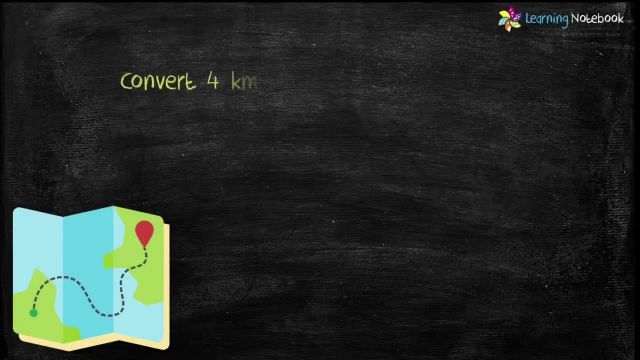 So half kilometer equals to 500 meter. Now let's do few questions. First question is: convert 4 kilometer into meter. Students, we just learnt to convert kilometer into meter, multiply by 1000.. So 4 kilometer equals to 4 into 1000 meter, which is equals to 4000 meter. 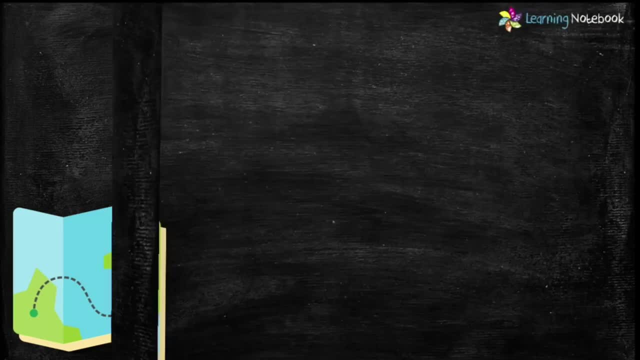 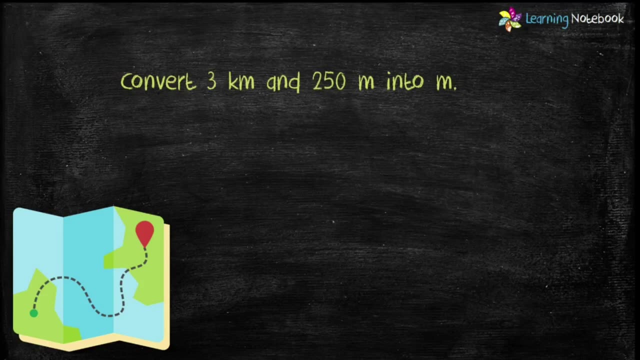 So to convert kilometer into meter we will multiply by 1000.. Next question is: Convert 3 km and 250 m into m Students, 3 km and 250 m means 3 km plus 250 m. Now we have two terms. 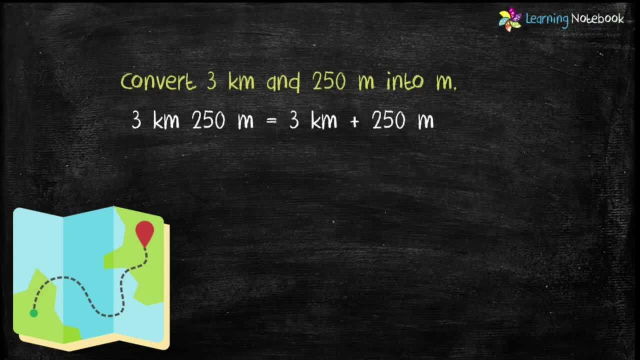 3 km and 250 m. 250 is already in m, So we will convert 3 km into m. To convert km into m, Multiply by 1000, Which means 3 into 1000, Which is equal to 3000 m. So, students, 3000 m plus 250 m. 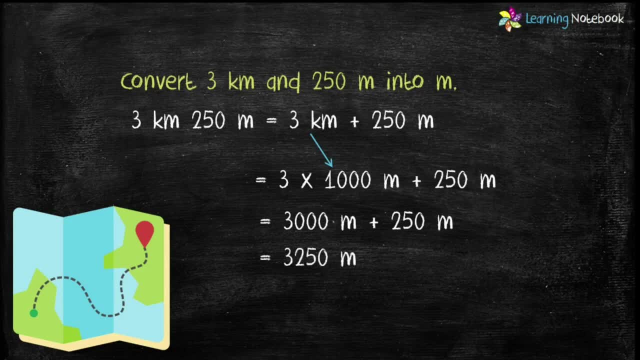 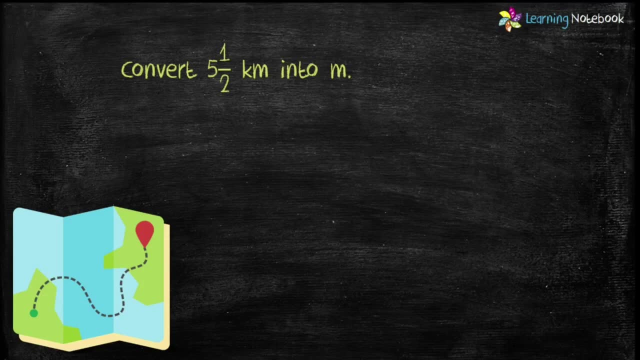 Which is equal to 3000 m, Equals to 3250 m. Let's do last question. Convert 5: 1 by 2 km into m Students: 5: 1 by 2 km means 5 km plus 1 by 2 km. 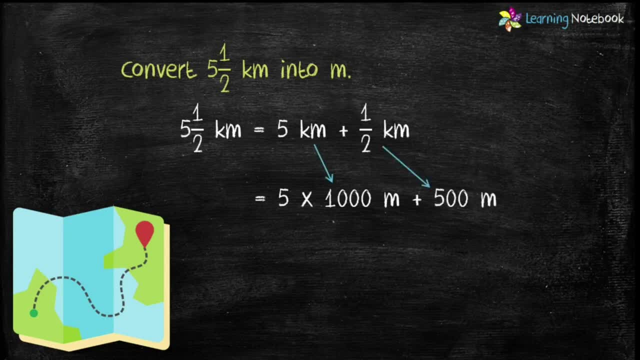 To convert 5 km into m, We will multiply by 1000, And half of that is 500 m. Therefore, 5 into 1000 m Plus 500 m, Which is equal to 5000 m plus 500 m. Therefore, answer is: 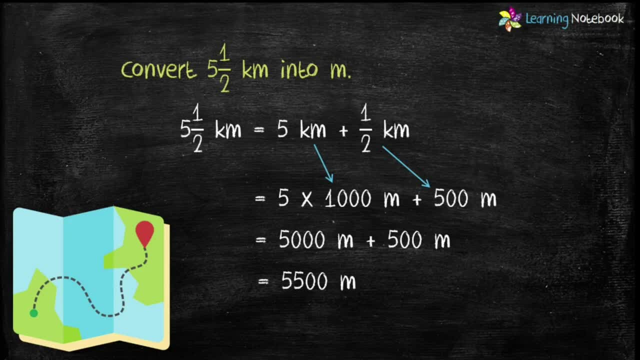 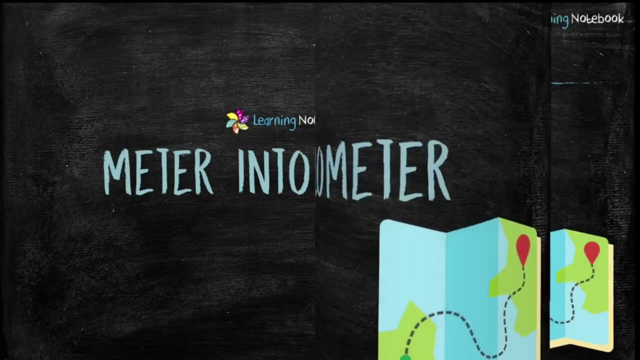 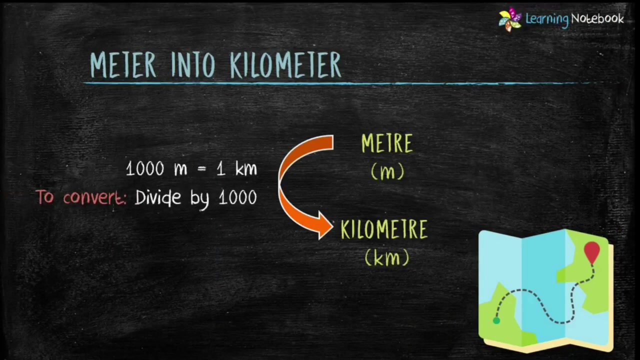 5500 m. So, students, this is how We convert km into m. Now let's see How to convert m into km. 1000 m equals to 1 km. So to convert m into km, Divide by 1000- And, students, we know, 500 m equals to 1 by 2 km. 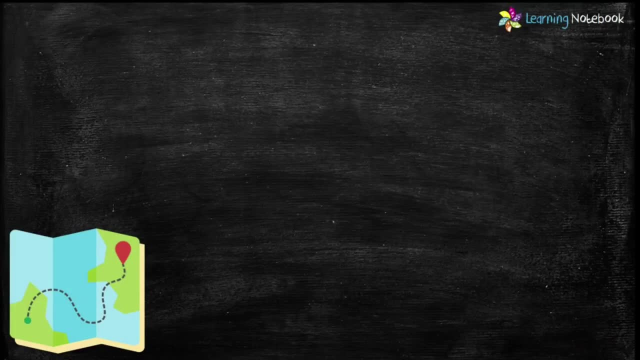 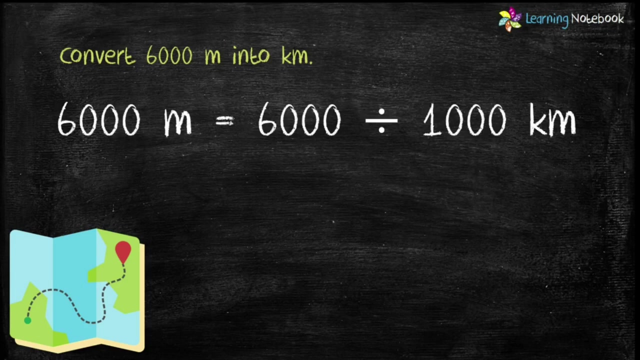 Now let's do Some questions based on it. Question is: Convert 6000 m into km. As we just learnt To convert m into km, We will divide by 1000. So 6000 m equals to 6000 divided by 1000 km. When a number is divided by 1000, 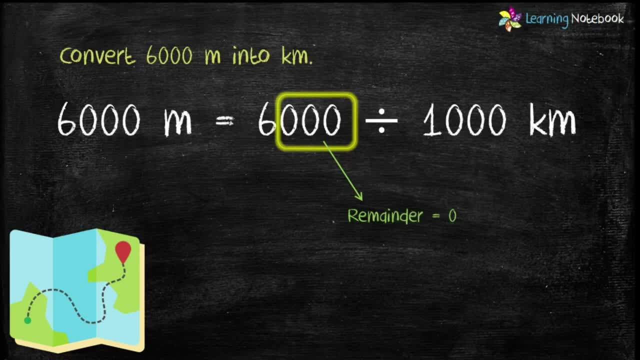 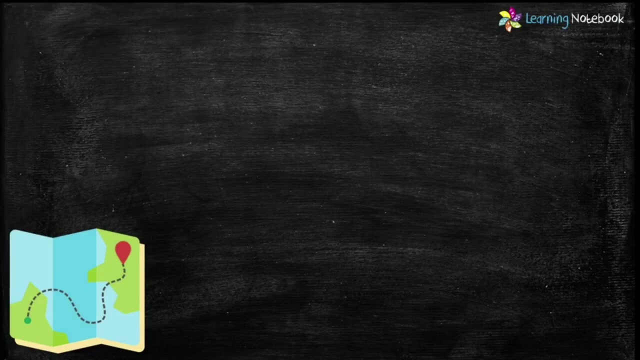 Digits at 1's, 10's and 100's place Make up the remainder. So here remainder is 0 And the remaining digits Make up the question. So here question is 6. Therefore answer is 6 km. Now next question is: 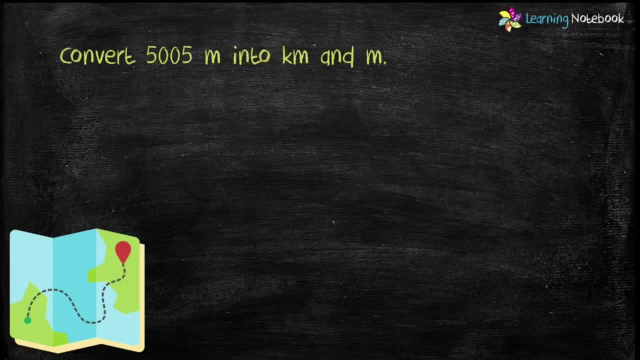 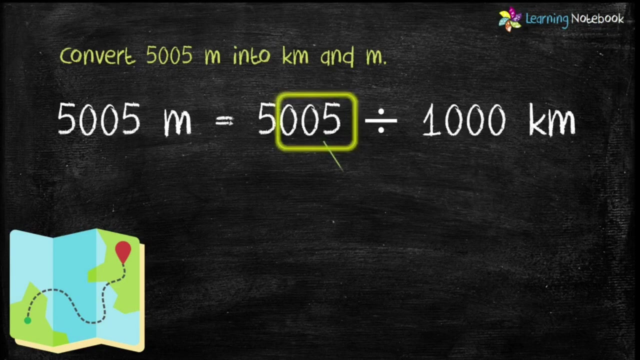 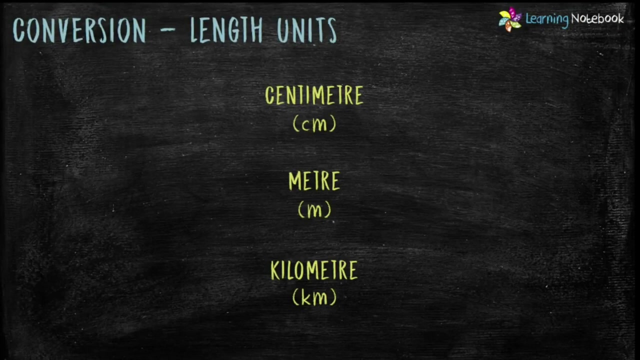 Convert 5005 m into km and m Students. to convert m into km, Let's divide by 1000. So here remainder is 5 And question is 5. Therefore, answer is 5 km, 5 m. Now let's summarize What we have learnt so far. 1 km equals to 1000 m. So to convert km into m, Multiply by 1000. Next, 1 m equals to 100 cm. So to convert m into cm, Multiply by 100. Now, 100 cm equals to 1 m. So to convert cm into m. 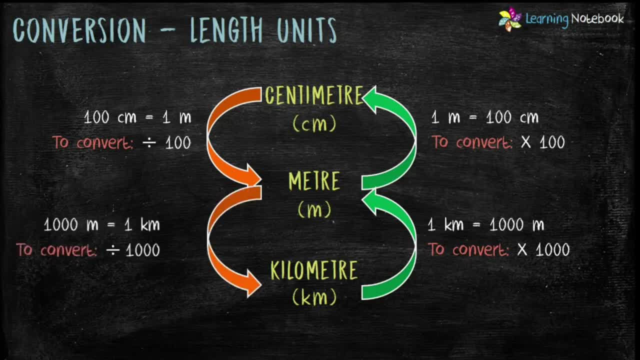 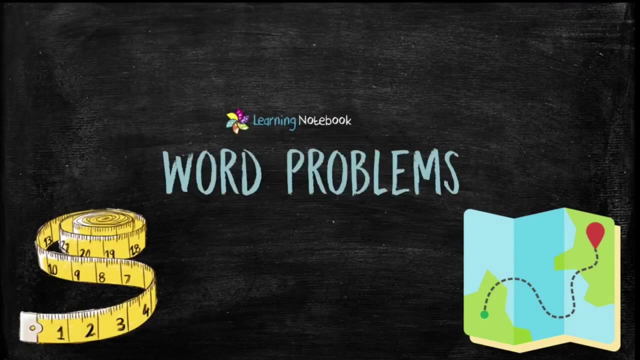 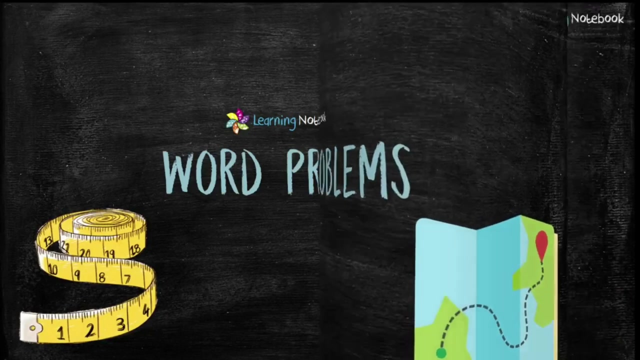 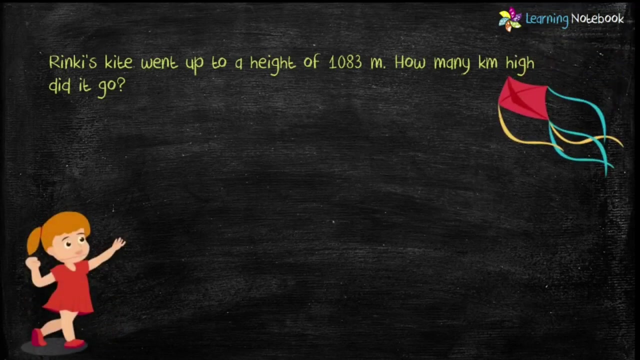 Divide by 100 And 1000, m equals to 1 km. So to convert m into km, Divide by 1000. Now, students, let's do few word problems Based on conversion of length units. First question is: Rinky kite went up to a height of 1083 m. 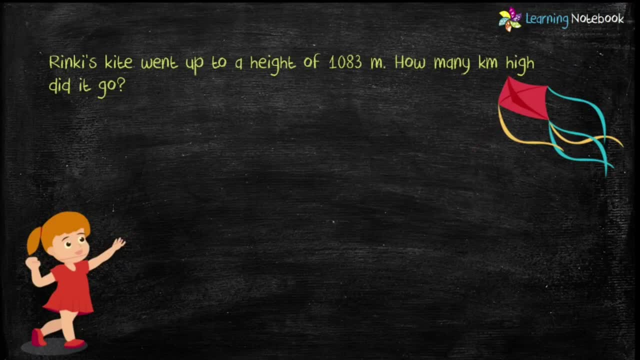 How many km high did the kite go? In this question we have to convert m into km, So it means we have to divide by 1000. So 1083 m equals to 1083 m Divided by 1000 km. So here remainder is 83. 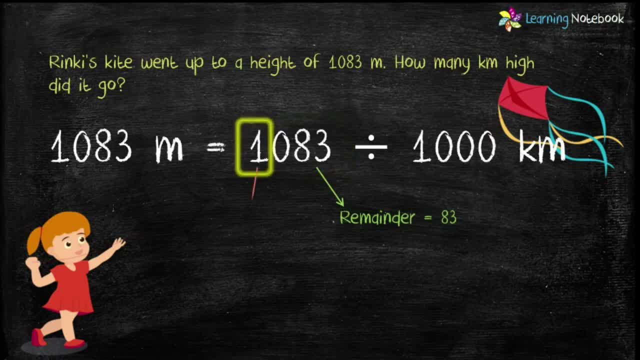 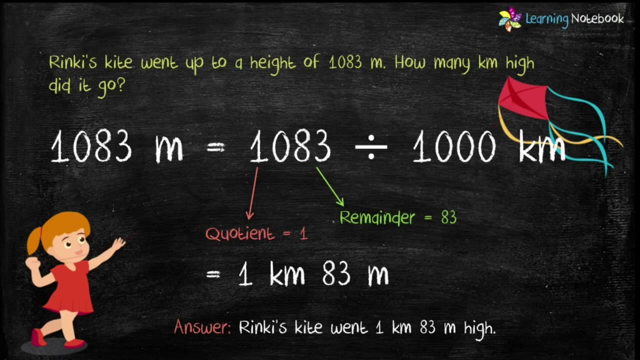 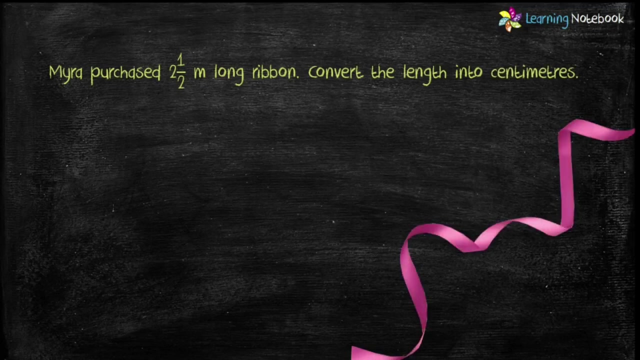 And question is 1. So answer is 1 km 83 m. Let's write the answer statement: Rinky kite went 1 km 83 m high. Next question is: Next question: is Myra purchased 2 1 by 2 m long ribbon? Convert the length into cm. 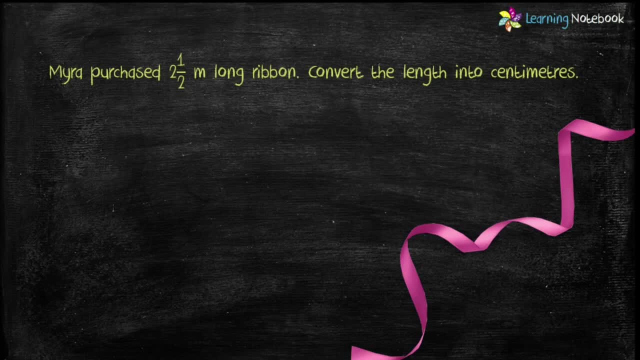 In this question we have to convert m into cm Students. 2: 1 by 2 m means 2 m plus 1 by 2 m. To convert 2 m into cm We will multiply by 100, And 1 by 2 m equals to 50 cm.